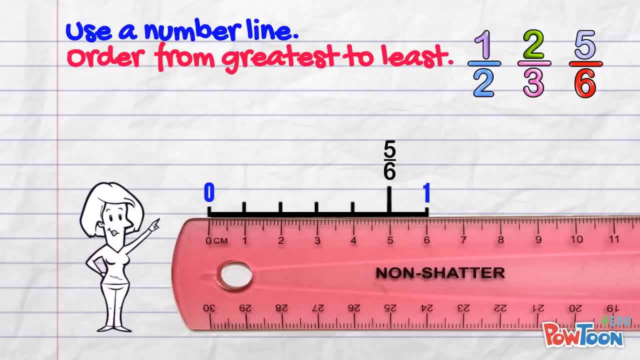 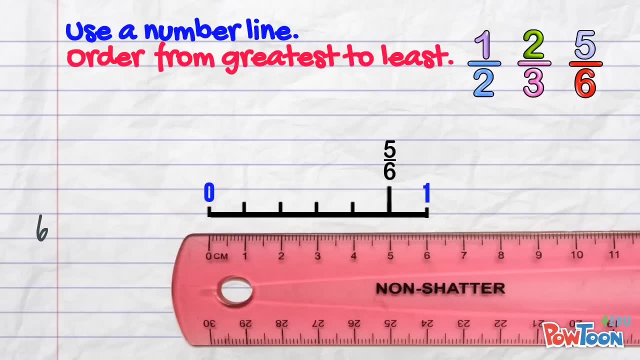 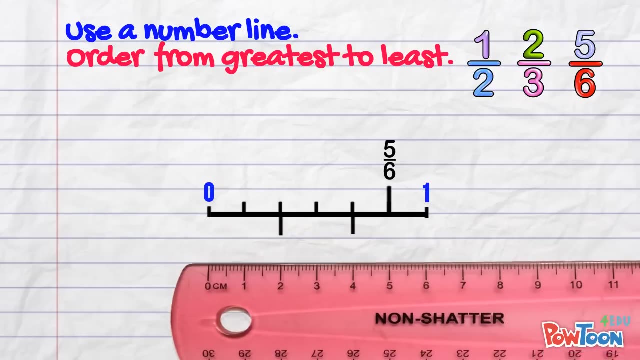 I mark it clearly On the bottom edge of the line I'm going to mark thirds. The whole line is 6cm and 6 divided by 3 is 2, so each third is 2cm wide. And here's 2 thirds. 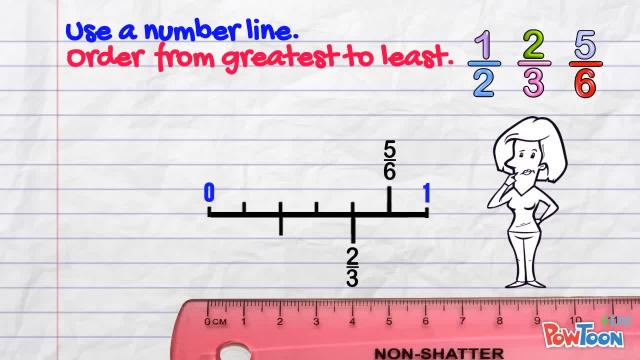 Again, mark it very clearly. And I still have to show 1 half. but I've used both edges of the number line. I've used the top edge for an even denominator and the bottom edge for the odd denominator. So now what I do is: 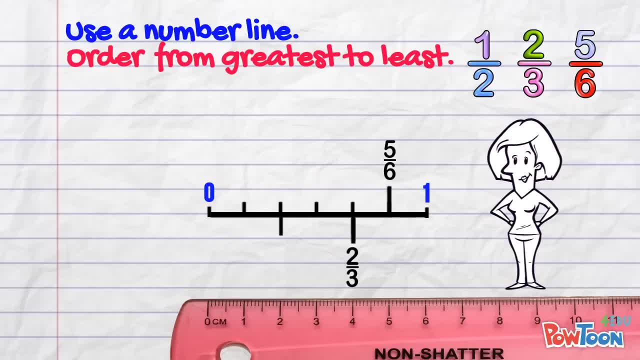 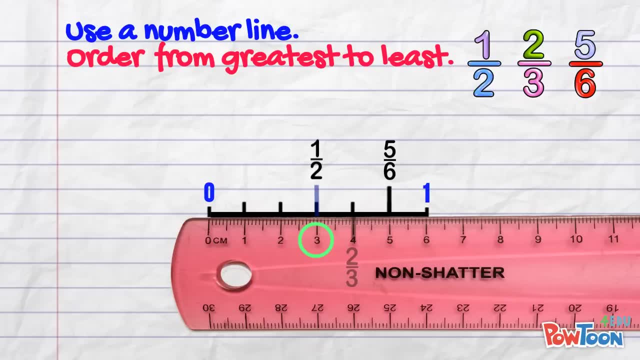 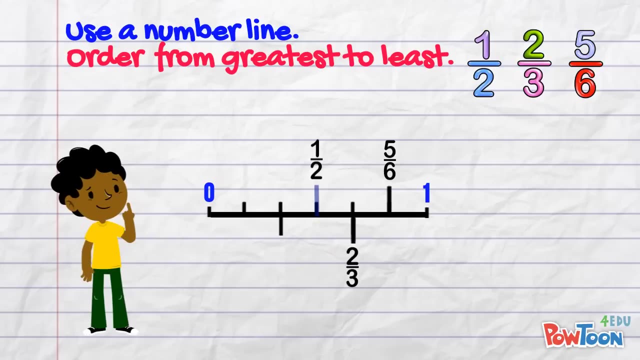 use a different colour. This helps me focus on what I'm doing with the colour right now. Half of 6 is 3 and here's 1 half. Maybe you're thinking What if I don't have a different colour? Well, not a problem. 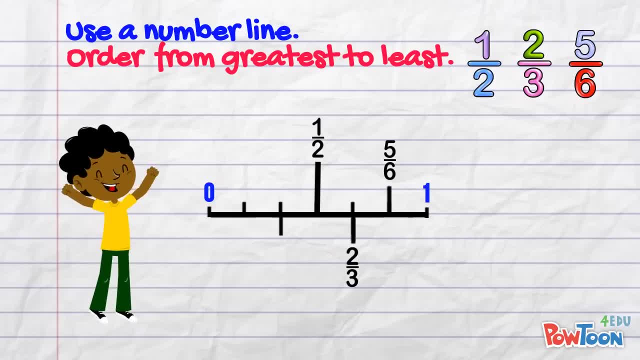 Instead you can just make a longer pencil mark so that it looks different from the other marker on the top edge. for 5, sixths, Making marks that look different. stop confusion when you look at the number line. With this approach, you could easily stack. 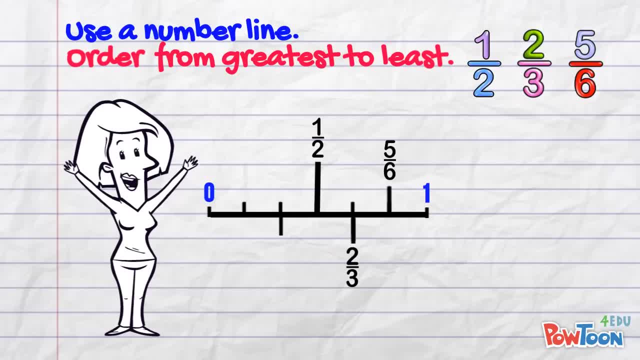 4,, 5 or 6 fractions on a number line. Ok, now we have to list the fractions in order from greatest to least. So start big and go small. Don't mess it up at this last step. First we write the fractions. 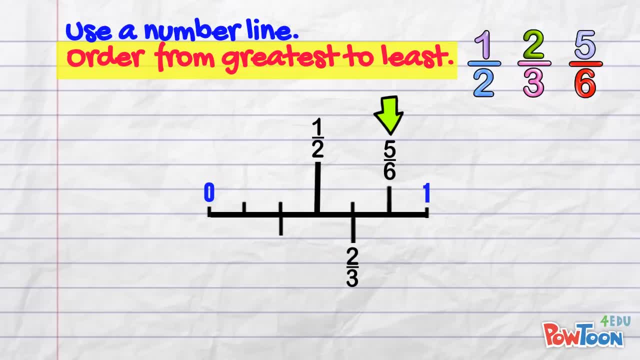 Look at the number line. The greatest fraction we marked is 5 sixths, Then it's 2 thirds, Then 1 half. Finally, we use the greater than sign to show our understanding: 5 sixths is greater than 2 thirds. 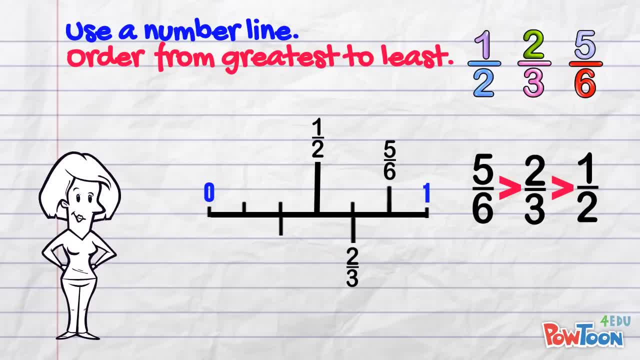 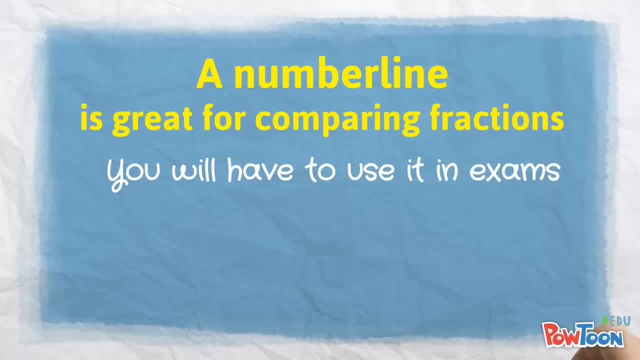 which is greater than 1 half. A number line is a great tool for comparing fractions, and you will have to use it in exams. You need to get comfortable creating your own number line as well as using one that's been made for you- The way to success. 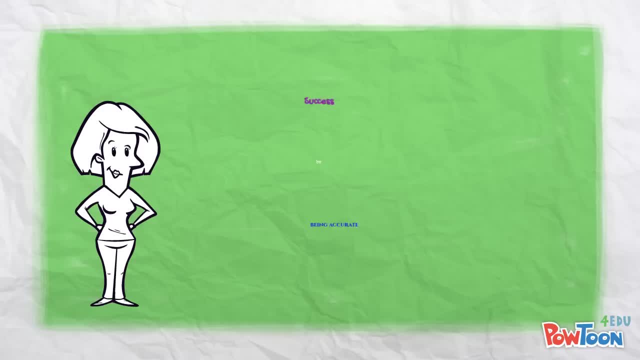 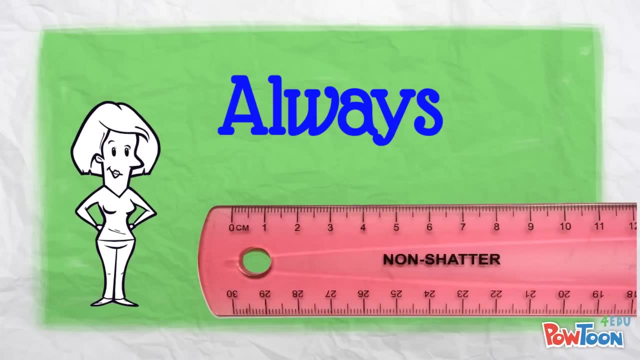 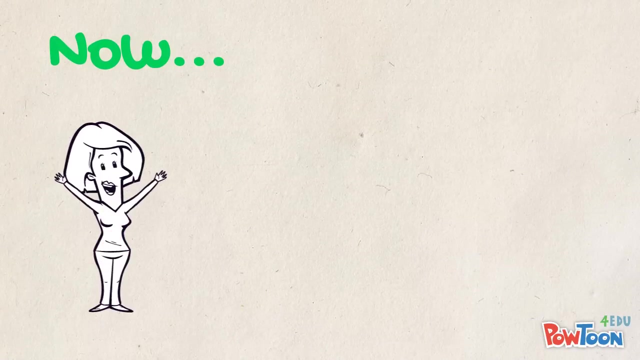 is by being accurate. So please never sketch a number line or guess it. Always use a ruler. Then the size order of the fractions is absolutely clear. And now it's your turn to work your math muscle. You're going to create your own number line.